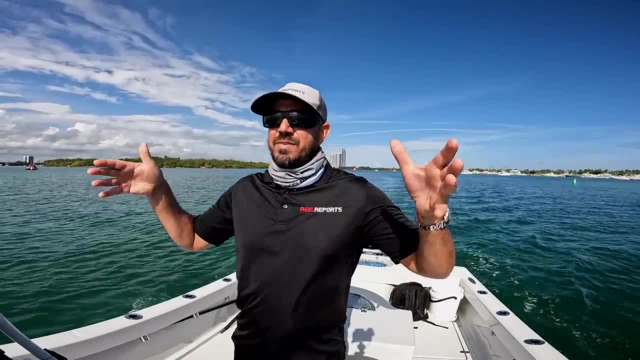 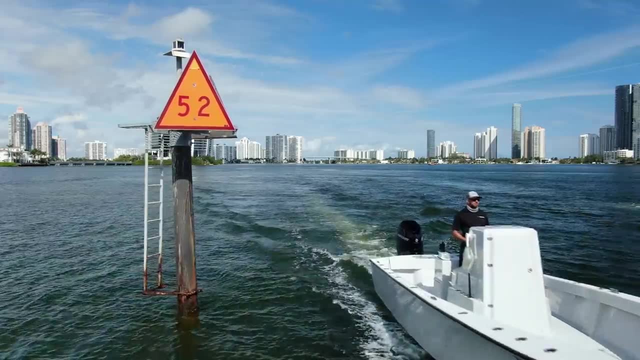 You don't want to go off into the sidewalk or into the grass. The same thing with the intercoastal waterways. here, They are marked by the United States Coast Guard to keep you in deep water, And this is especially important when you're on a big boat. However, down here in Miami, 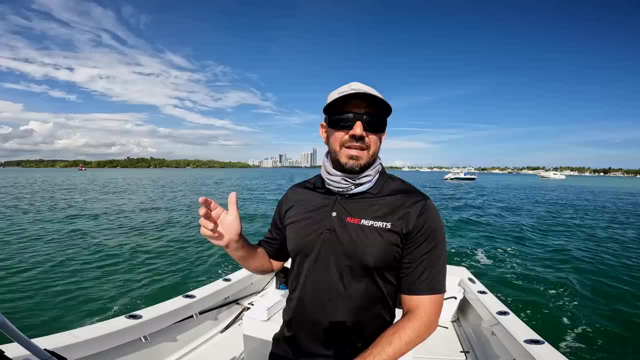 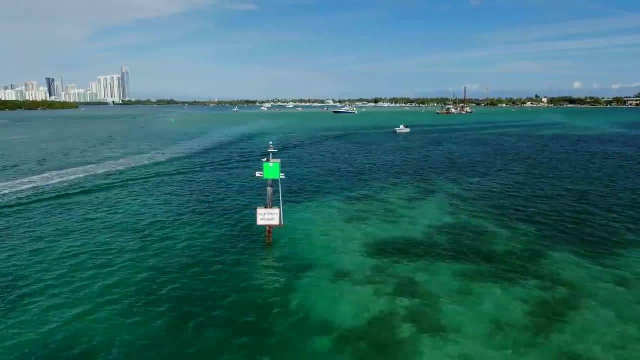 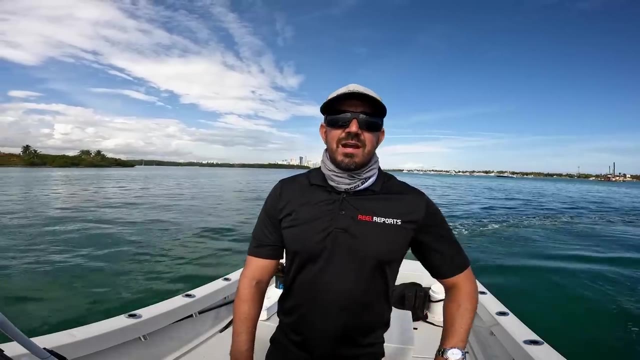 where I'm at right now- big boat, small boat. you could easily run aground here, which means you'll go in water too shallow for your boat and you'll end up stuck or, even worse, damage your motor or even hurt somebody. So we want to make sure that we do none of that. The first concept that I 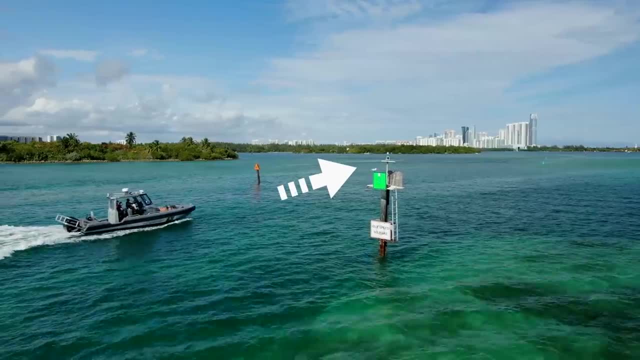 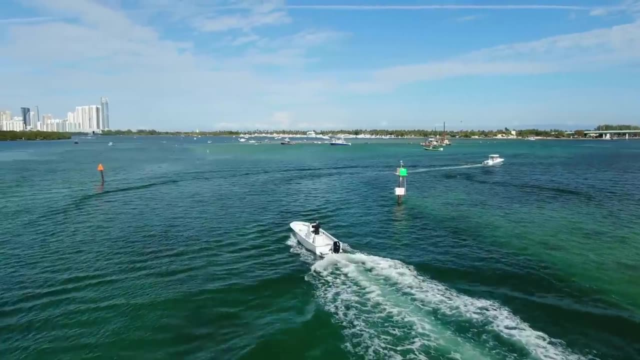 want you to grab is if you see a red and a green channel marker. we have a saying in boating: red and green stay in between. A lot of the times there's tight channels, just like this one, where you're able to see both the red and the green pretty much right side by side. Get in between. 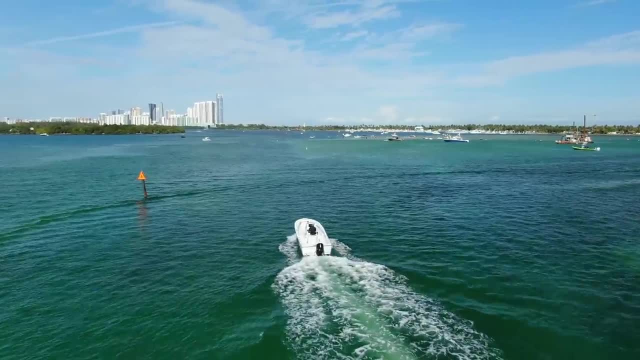 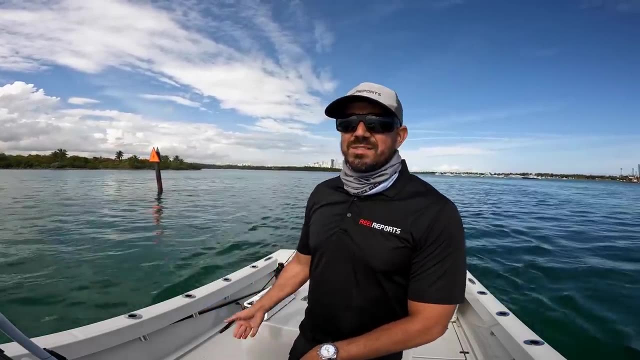 those. That's the easiest form of navigation. Now, a lot of times you won't see both channel markers side by side like that, In fact most of the time- So you want to make sure that you're. you have to know what side of the boat the red one should be on and what side the green should. 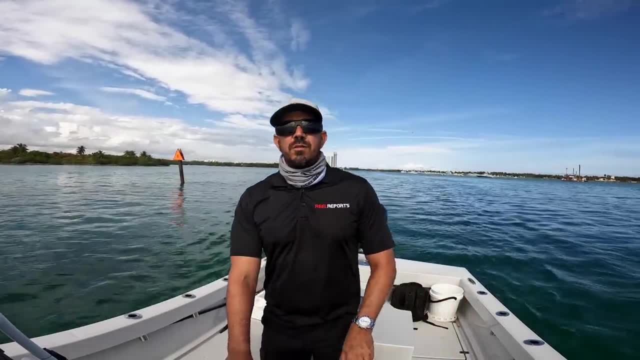 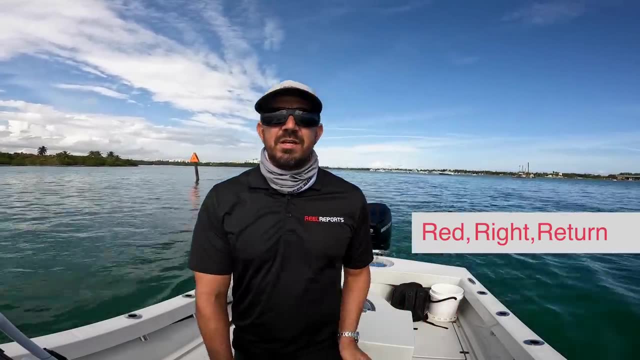 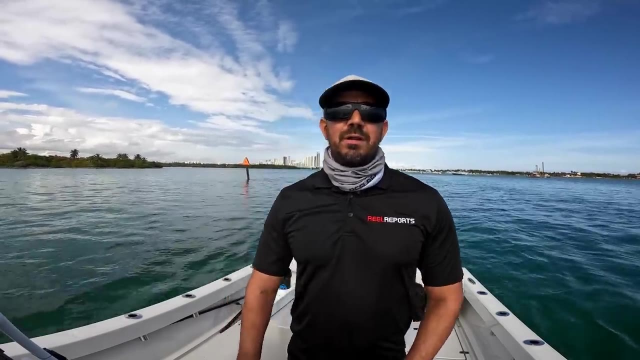 be on. So here's another term that I want you to remember, Another phrase that we say: red right return, Red right return. They call it the three R's. It is boating 101. Remember that. So what that means is, anytime you're coming from an open body of water, that is when you're coming off the 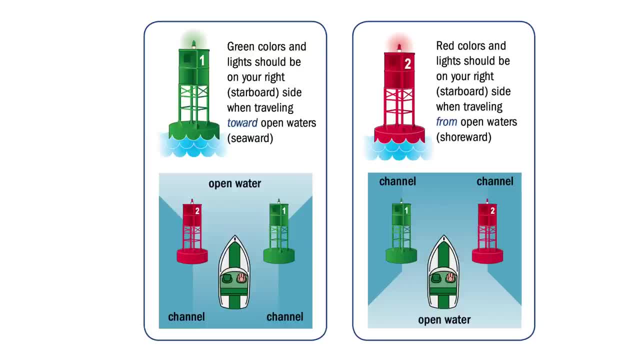 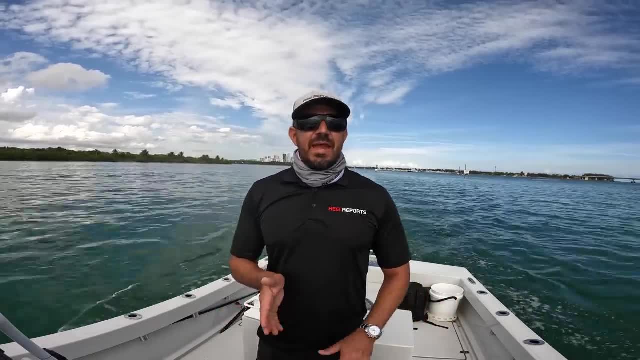 ocean. coming into your home port, the red is always going to be on your right. Red right return, which means the green will be on your left. When it comes to navigating the intercoastal waterway, the Coast Guard gave us dayboards. These are little yellow squares and 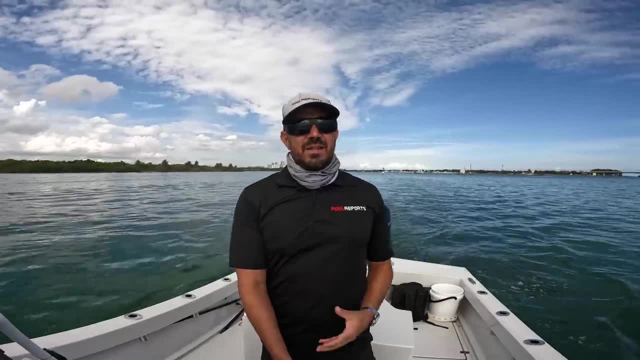 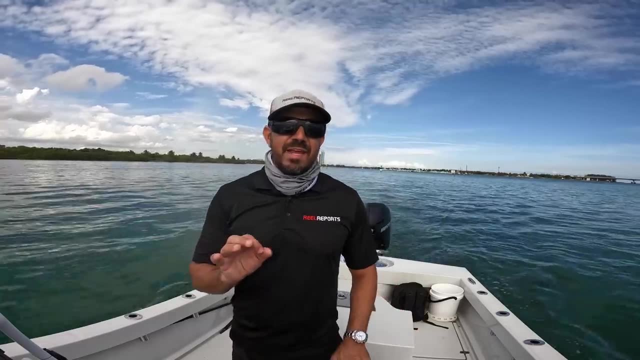 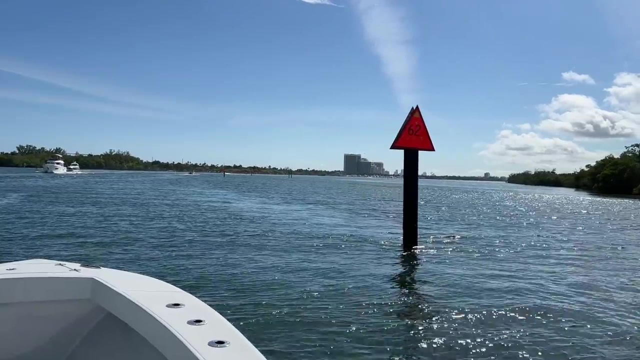 triangles that they place on navigable instruments. They might not always be on a typical channel marker, So what they're on doesn't really have significance. The important thing is that you know what to look for and what side to keep them on. So the red right return rule does apply. 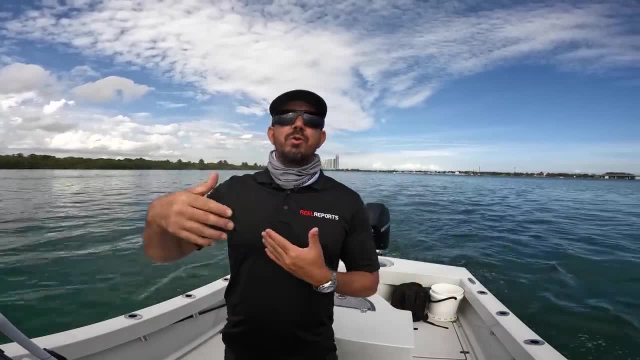 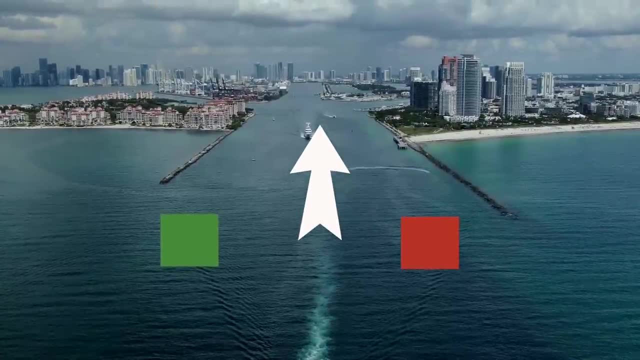 to the intercoastal waterways as well. But you got to know what your port is. When you're coming off the ocean, it's obvious that you're coming into port, So you're coming from an open body of water. Red right return. Keep that red channel marker on your right. Well, when you're going, 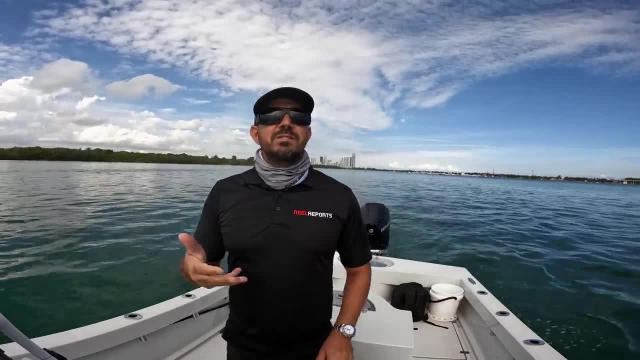 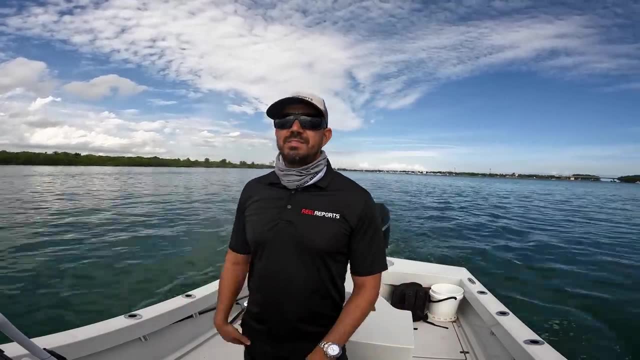 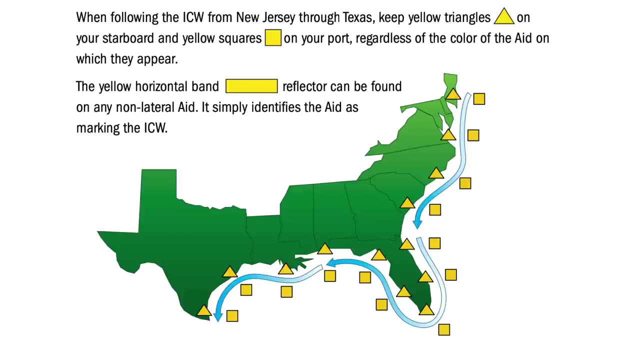 from New Jersey onto Florida. where is the home port? That's what's going to determine which side those dayboards are going to be on. The Coast Guard makes it easy for us Pretty much: if you're from New Jersey to Texas, to Florida, you're heading in that south, that southerly direction. 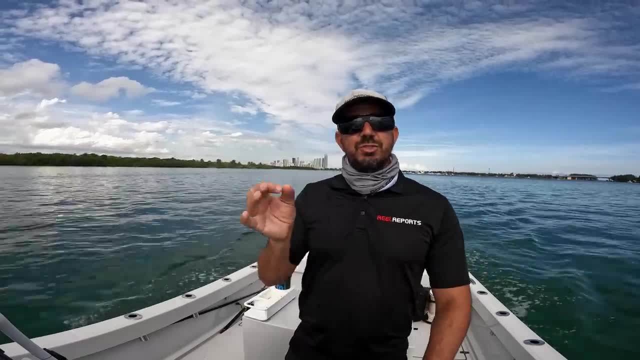 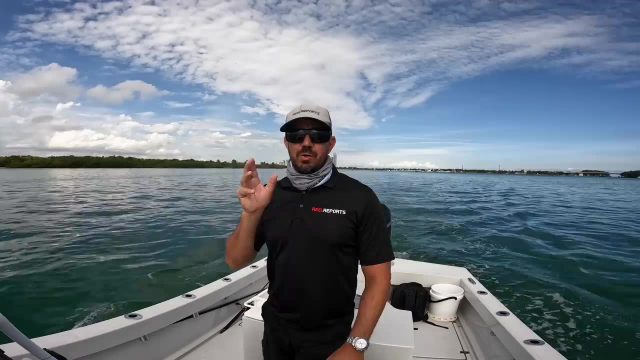 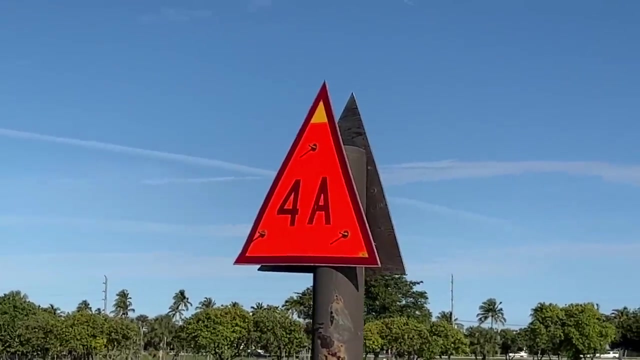 You're going to be looking for those squares and triangles on those channel markers or on you know some sort of beacon out there. So know your port. So I'm heading south here. I'm in Miami, Let's just say I'm heading to the Keys. The triangles are always going to be on my right. 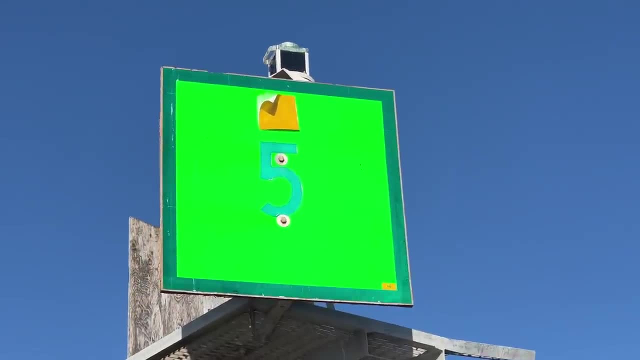 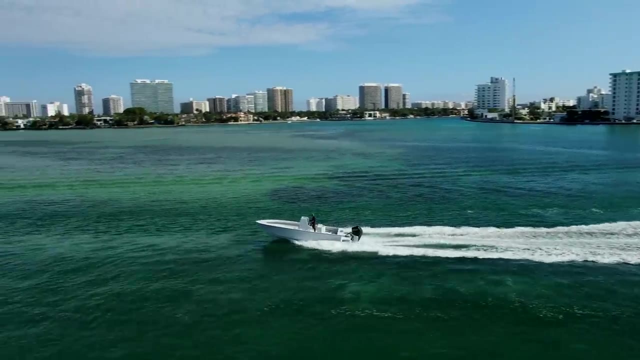 and the squares are always going to be on my left or my port side. That's key. Now, if I was heading from Miami up to Virginia and go pick up my dad up there and do a little cruising around, I would have to do the opposite. The triangles are then going to be on my left. 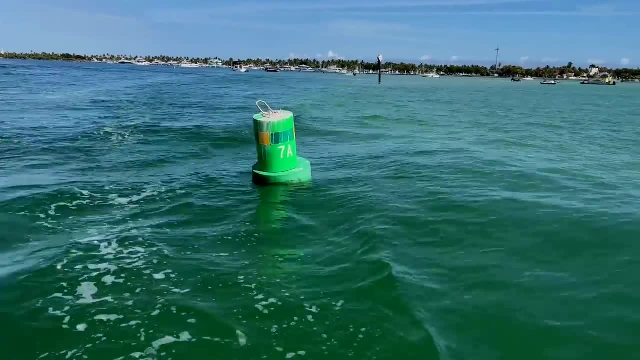 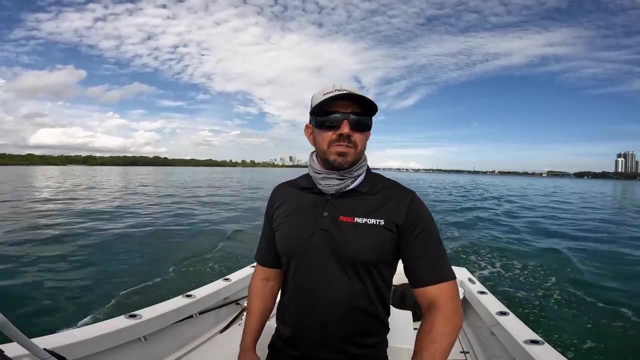 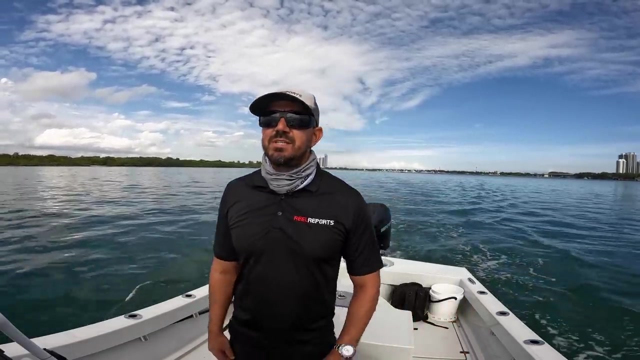 and the squares are then going to be on my right or my starboard. The color really isn't of importance, because the United States Coast Guard knows that a lot of us are colorblind, So you're looking for the shapes. Shapes are what you can see a lot easier in the 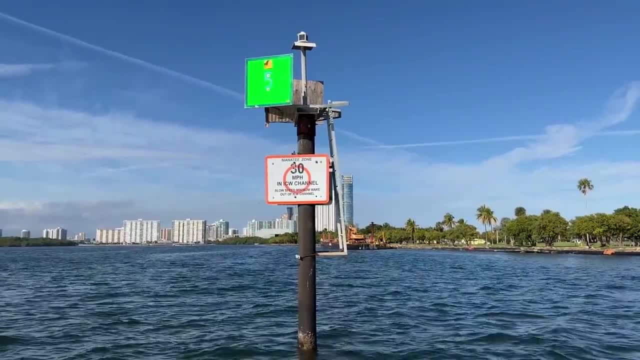 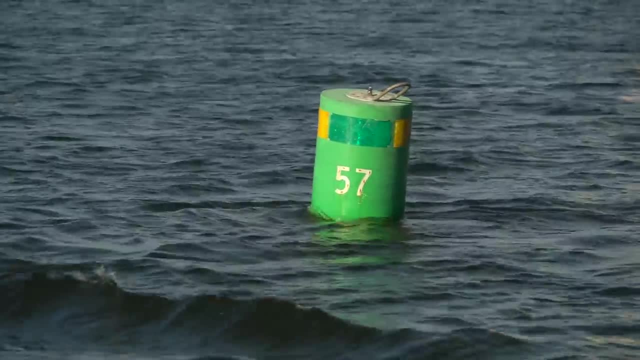 coaster. You get to them, you'll be able to see that. Just remember that the day markers are of the most importance when you're traveling through the intercoastal waterway. You want to pay attention to those little squares and triangles on these aids to help you better navigate and 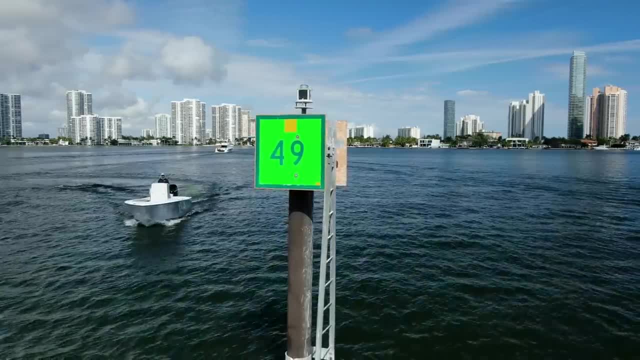 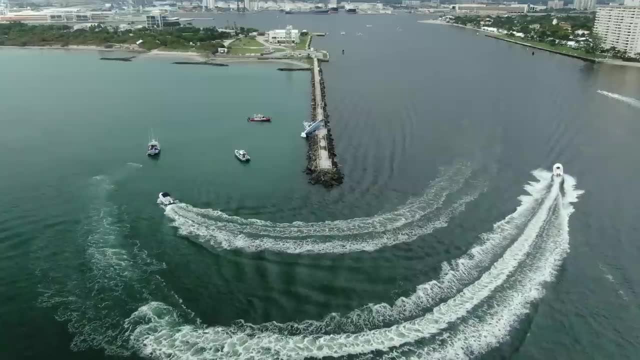 stay in the channel. When you go out of the channel you risk running aground, damaging your prop, damaging your boat, or somebody could even get hurt. So it's of your best interest and your responsibility as a captain of your boat to know how to navigate the waterway. So if you're 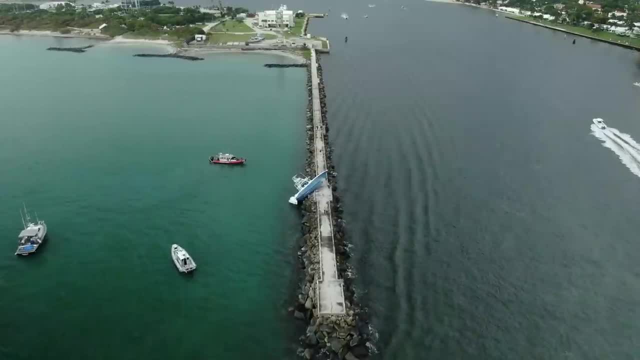 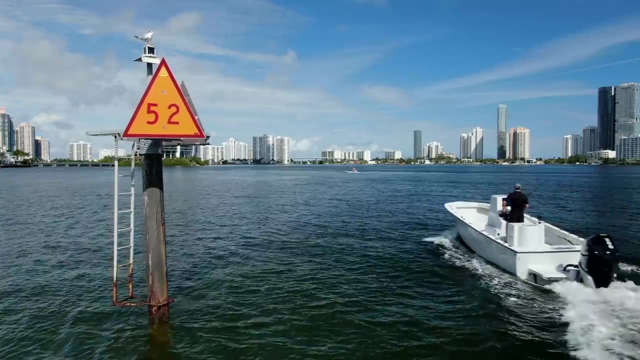 going to be out of the channel. you're going to want to know how to navigate these channels, And that's exactly why they're here. The Coast Guard put them here so you can stay in deeper water, And this specifically applies to all size vessels. I don't care if you're in like a, you know, an eight. 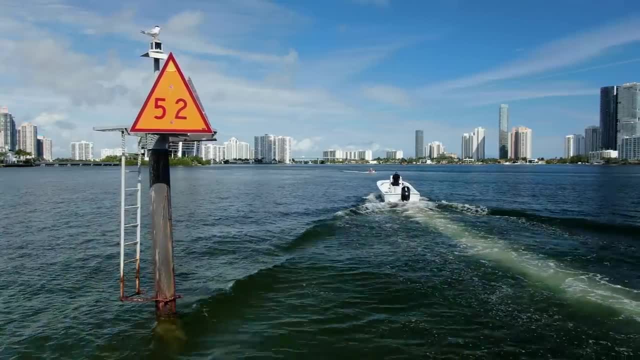 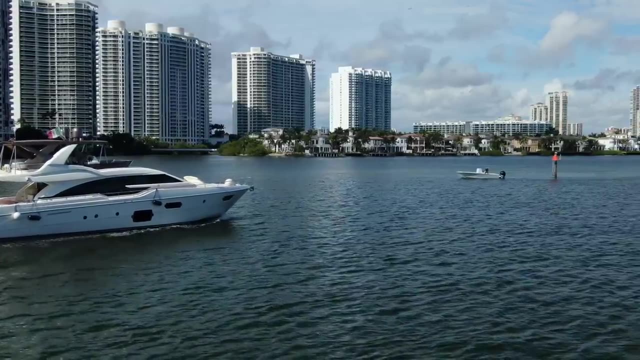 foot boat. All right, And now that you know how to safely navigate the channel, I can sleep better at night, knowing that you and your family are going to be safe out there and you guys are going to have a great time on the water. Just remember, when you venture outside the channel or accidentally- 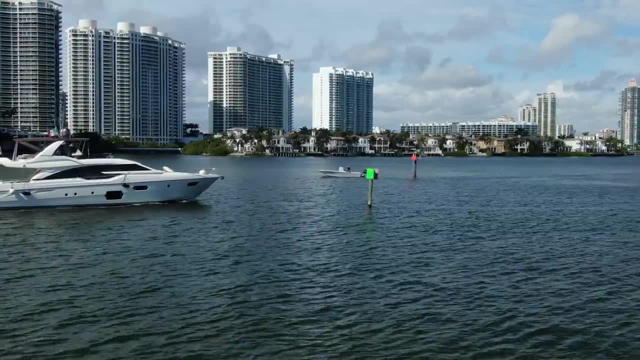 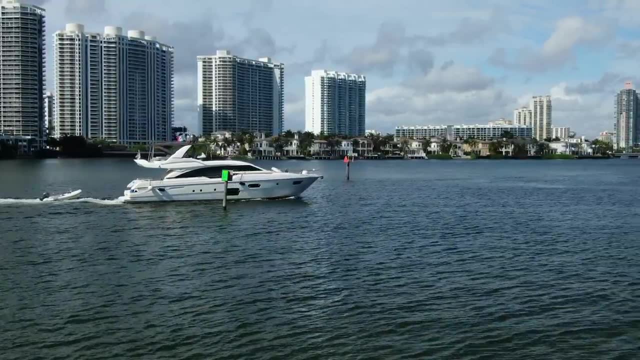 get out there, you do risk running aground, damaging your boat or somebody could even get hurt. So knowing this stuff is your responsibility as a captain. And it's super easy. Remember the saying: red right, return red and green, stay in between. Those little things will save you, But even 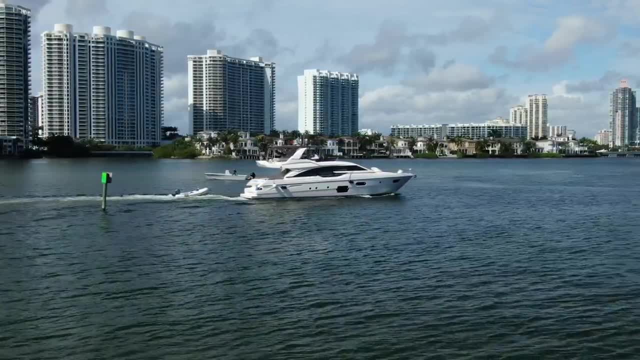 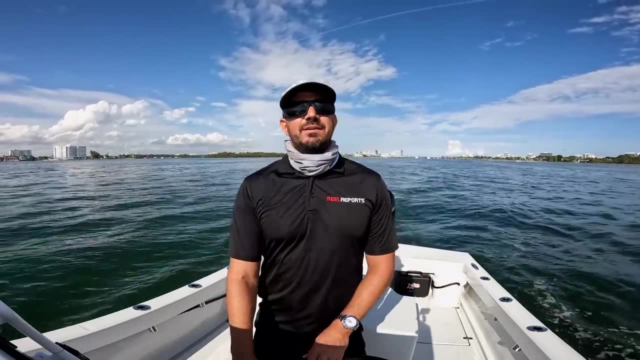 knowing more, knowing what they mean, is going to help you. So I can't do a video without giving something away. So we're going to give away something from LiveBaitcom, We're going to give you a t-shirt and we're going to do a pop quiz for it. I want to know how much you learned today. 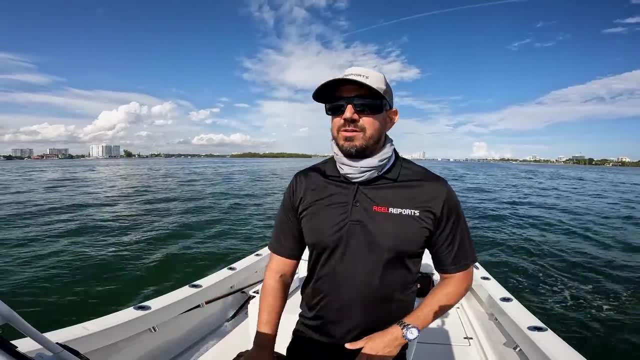 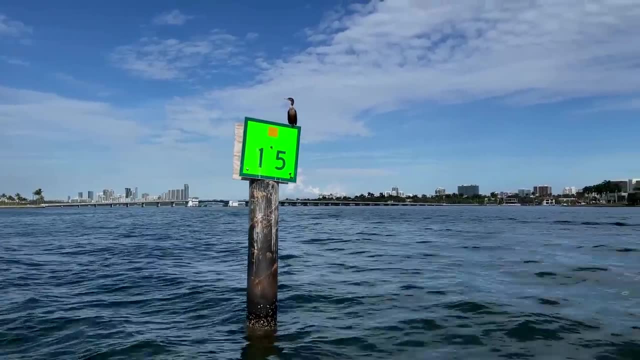 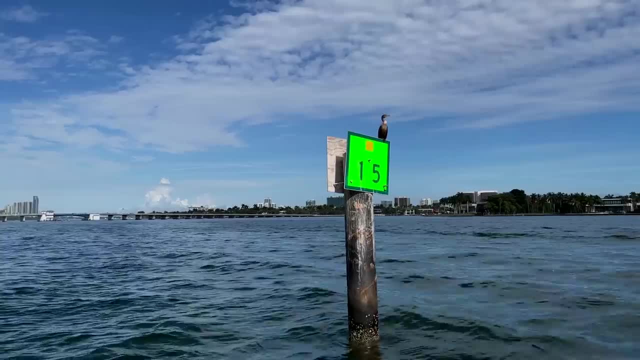 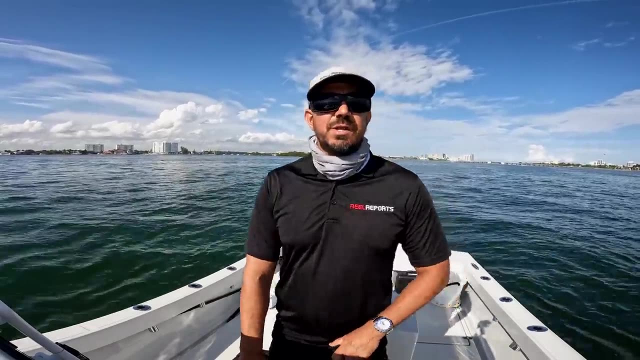 to my home. Which side of the boat should that channel marker be on Comment below and tell me why I'm going to pick a winner in the comments. We're going to send you something from LiveBaitcom, So I hope this reaches the right people. Please share this with your family. 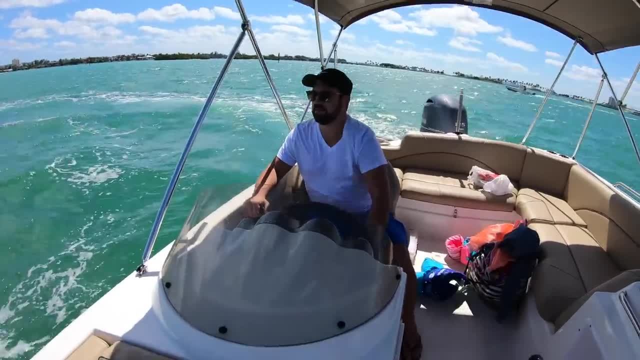 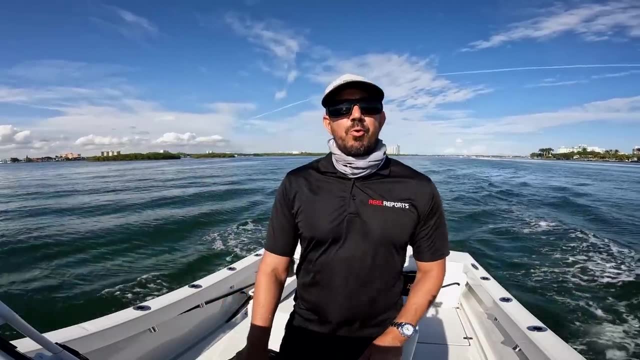 your friends If they're new to boating. this is something that everybody needs to know. This is going to help you have better days on the water, safer days out there. My name is Captain Mike. This is Real Reports. Take care of your neighbor. We're all in this. 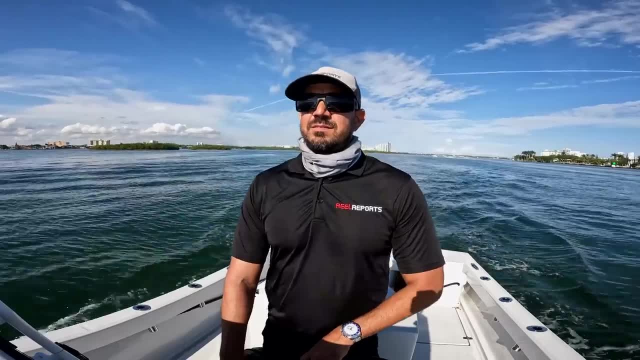 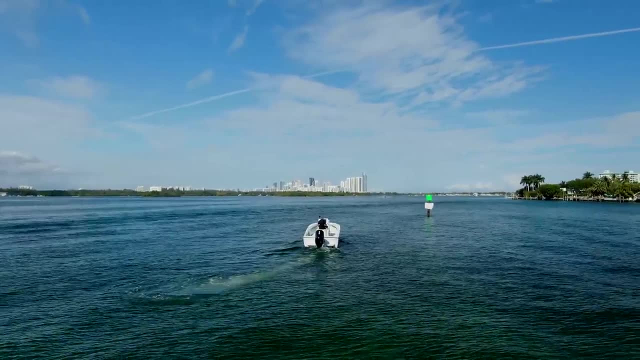 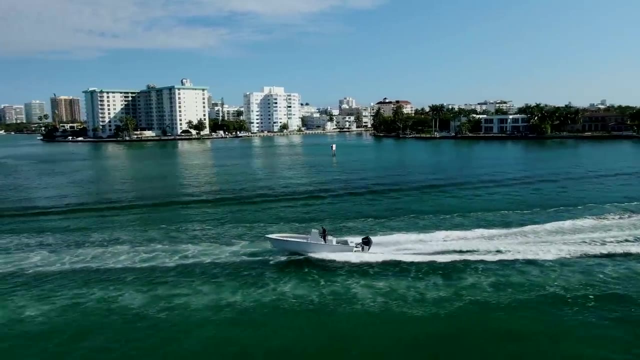 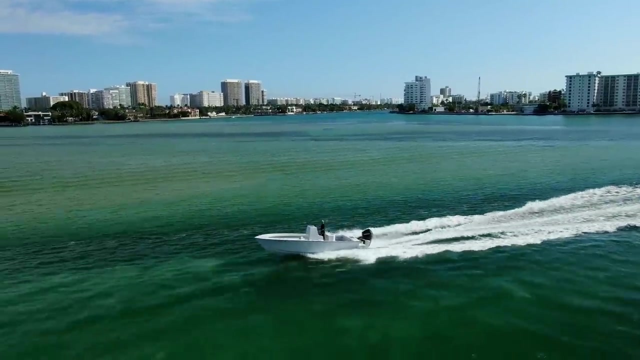 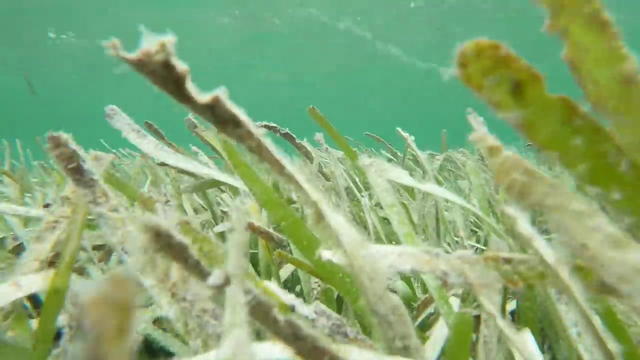 together. Have a great day everybody. By staying in the channel, it's also an act of conservation. When you verge outside channels a lot of the times, there is natural seagrass over there, which is extremely important to our ecosystem, And when you chop that up with your propeller, 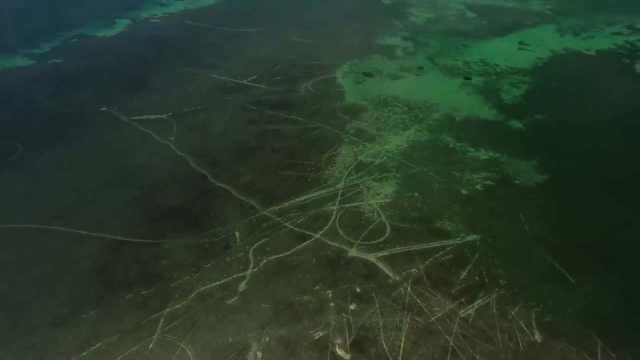 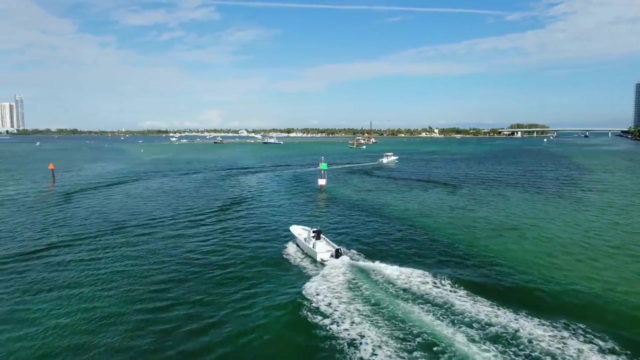 you're damaging, you're ruining that habitat for all those micro bait fish that in turn become bait fish and even bigger fish and so on and so forth. So by staying in the channel, you're doing your part on conservation, which is a huge thumbs up here at RealReportscom.